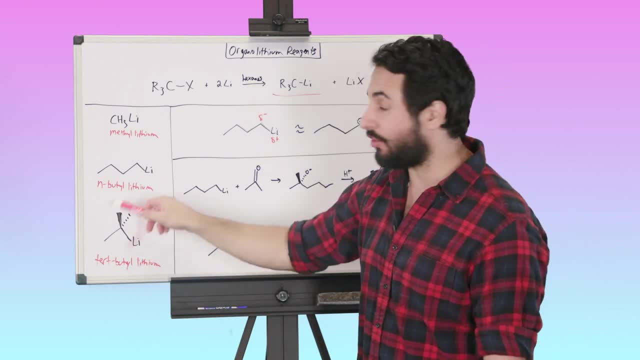 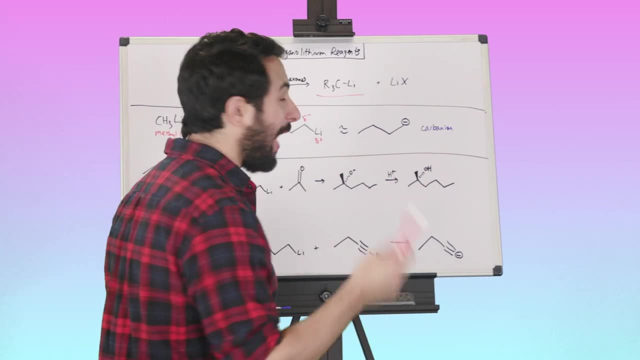 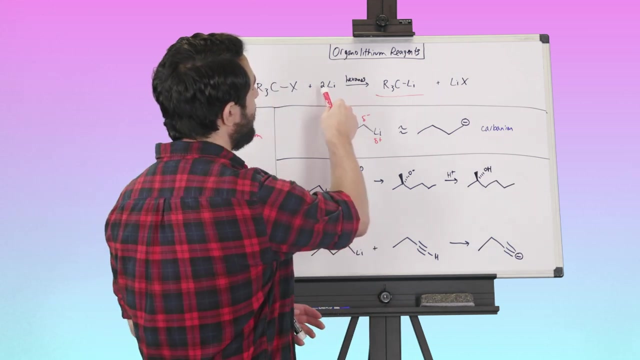 tert-butyl lithium. So here's a lithium and this is essentially a tert-butyl group. So these are three probably the most common organolithium reagents. And so what are the properties of organolithium reagents? We remember when we looked at the Grignard reagents. right, this is a bit. 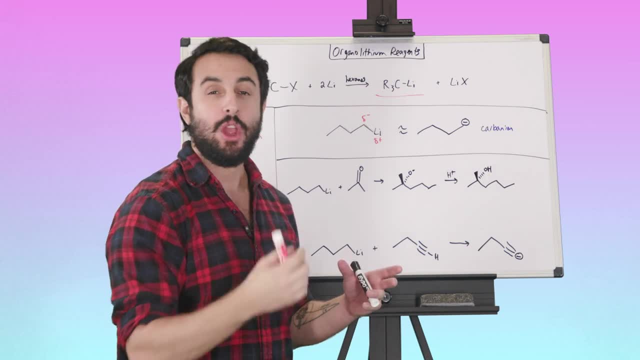 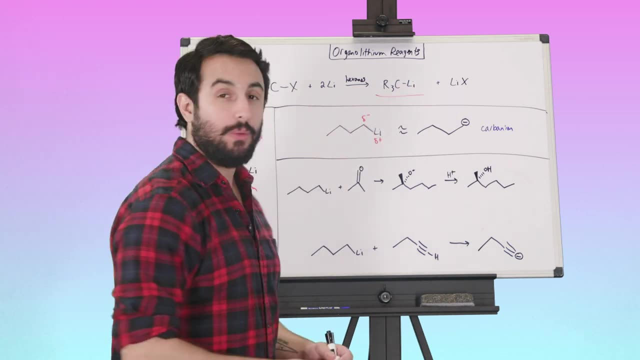 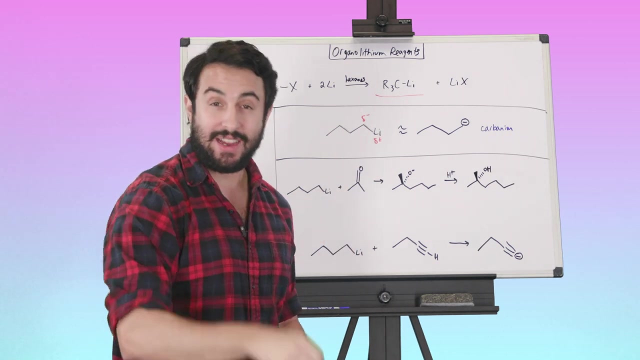 different, because we saw that the magnesium atom would insert itself into that carbon-halogen bond, whereas here the lithium simply displaces it. So we don't have that halogen anymore, we just have lithium, And as it happens, lithium is even less electronegative than magnesium. So 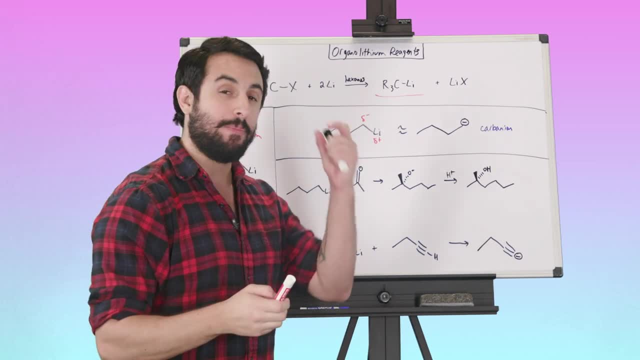 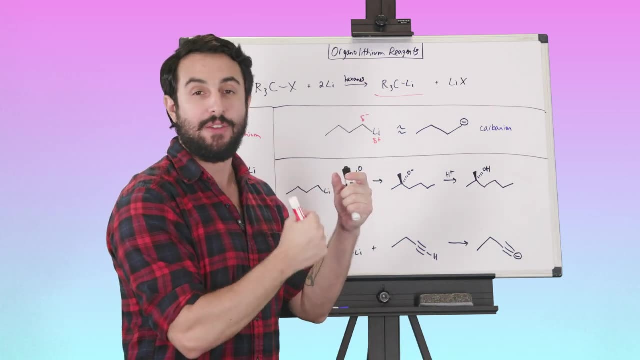 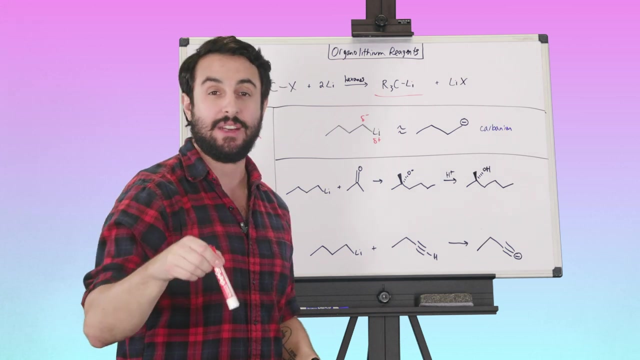 whereas with the Grignard reagent we saw that we had a partial minus charge on that carbon because it was a polar bond and carbon was pulling electron density away from magnesium. here we see that effect even more so because lithium is less electronegative than magnesium. 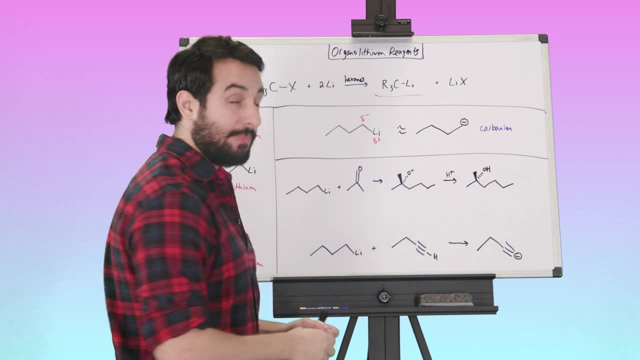 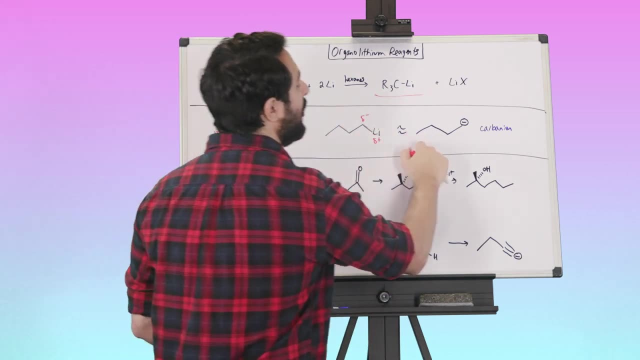 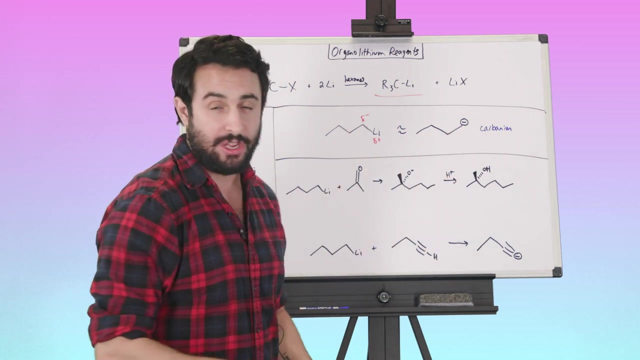 So this is an extremely polarized covalent bond. This is an extremely- this is a very significant partial minus charge on the carbon, so much so that this behaves almost like a carbanion. It is almost as though this carbon has a formal negative charge And, of course, 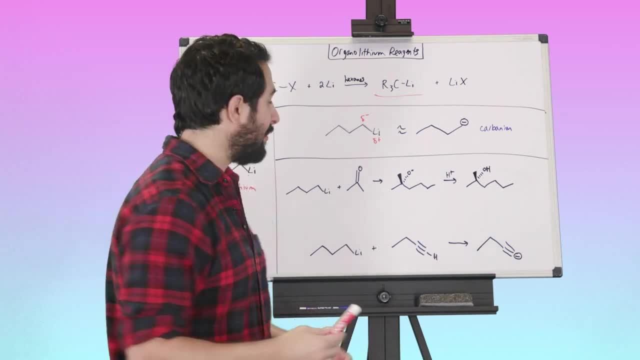 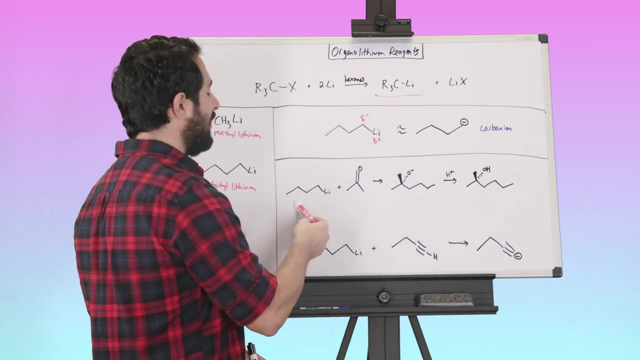 we know that. that means that it is extremely reactive as a species. So what are some things that we can do with these organolithium reagents? One very common thing is that these are just sources of nucleophilic carbon, again very much like Grignard reagents. So here's n-butyllithium. 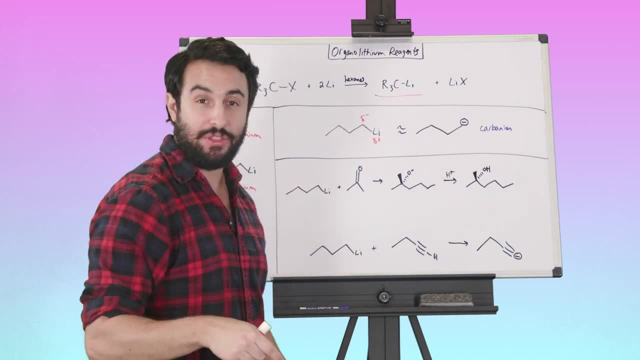 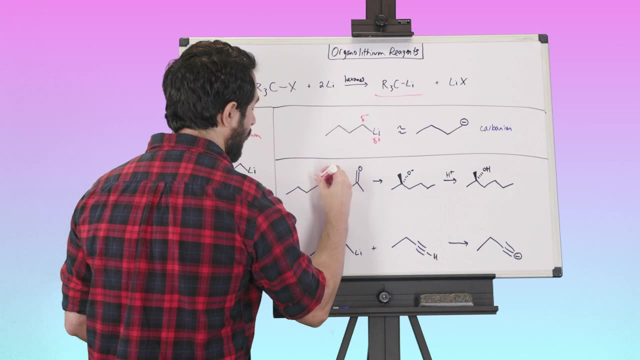 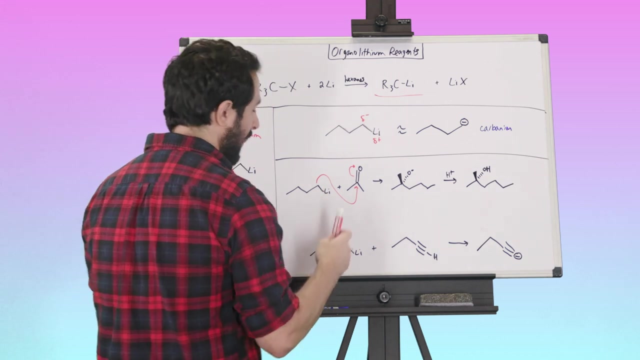 and remember that this carbon attached to the lithium is the one that bears that very strong partial minus charge, almost like a formal minus charge. So this is clearly the nucleophilic carbon. So that can come up here and attack a carbonyl just like a Grignard reagent. And now we've got 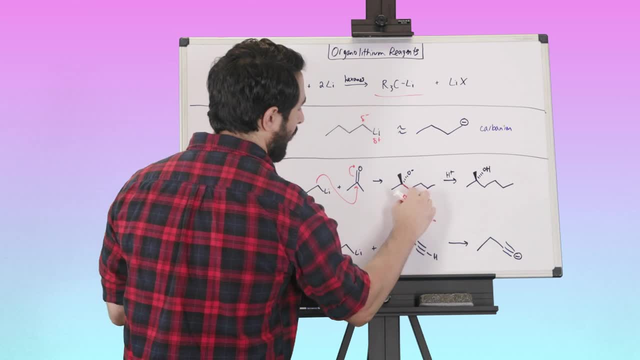 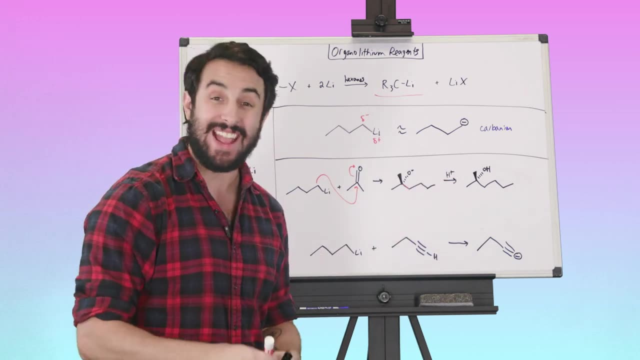 so this is the bond that was formed right here. right, We've got one, two, three, four carbons, that's those four carbons, and then these two carbons are right there and we've got that oxyanion, And then, of course, we've got the nucleophilic carbon, and then we've got the 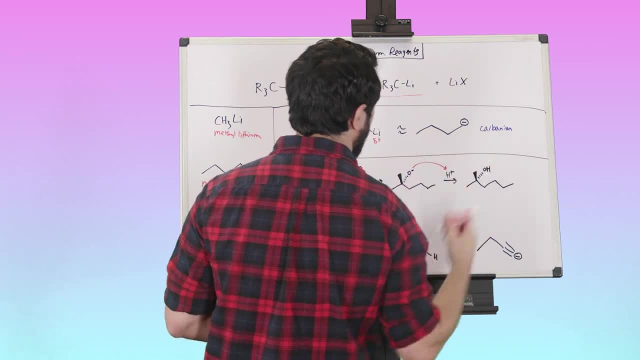 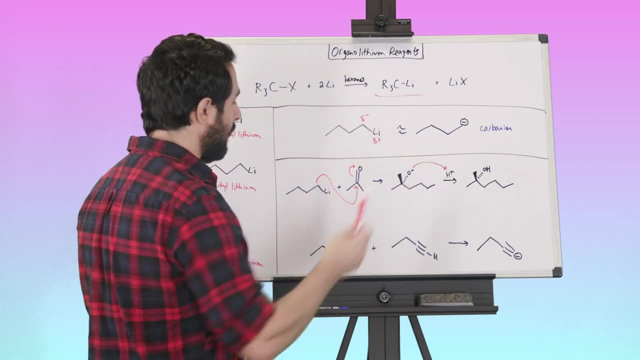 nucleophilic carbon And then, of course, any kind of acidic workup ammonium chloride. what have you? we're going to be able to protonate and we're going to get our alcohol. So this is extremely similar to Grignard reagents. We could also do that with a Grignard reagent and might want to.